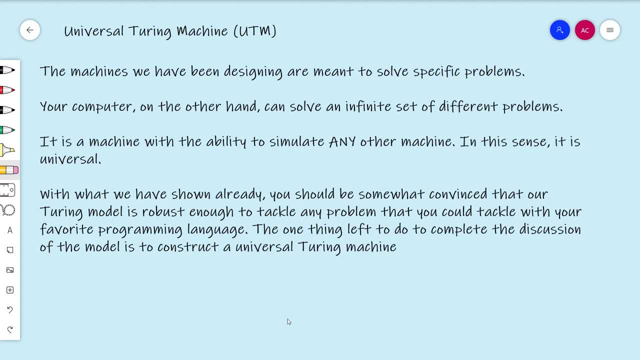 And hopefully I don't even need to do that. Hopefully you can just see that there would be a way to deal with that, There would be a way to mess around with that and make it work. So it's exhaustive in that sense. Another sense in which the model is exhaustive is that its initial premise, its initial promise, was that it was the kind of 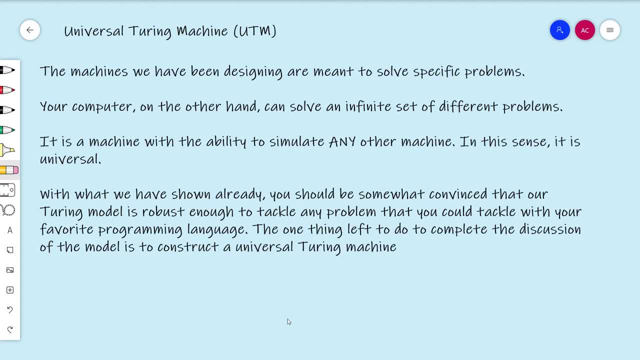 you know, formalization and sort of captured the essence of the idea of a person with paper and a pencil, thinking and writing on a paper and interacting with those things that he's written down. right, It was the original idea, was a very natural one in terms of not capturing the idea of a computer, but an idea of just algorithmic thought as a whole. 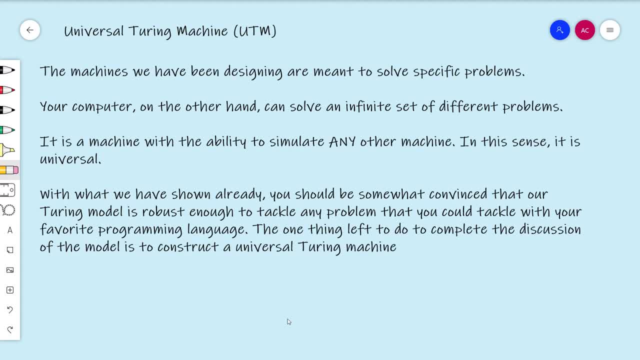 And so you know, given those two things combined, you should be somewhat convinced that this Turing model is at least robust enough to tackle any problem that you could tackle with your own favorite programming language. If you can do it in C, if you can do it on paper, if you can do it however you want, then you can probably make a Turing machine that does it. 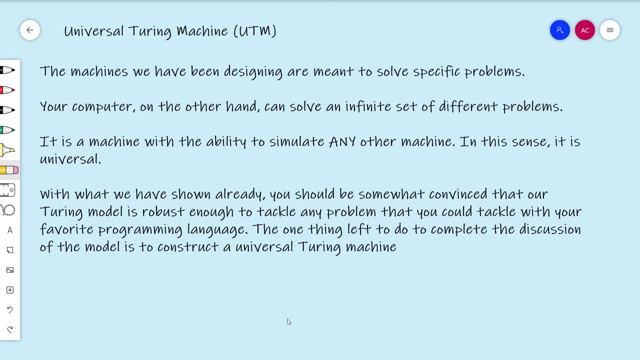 Hopefully I've convinced you of that through this exhaustive kind of- admittedly boring- collection of lectures so far, But I felt like it was important to do that. The one thing we have left to do is we need to make a universal Turing machine. So, even despite all of that, even despite its potential for problem solving, 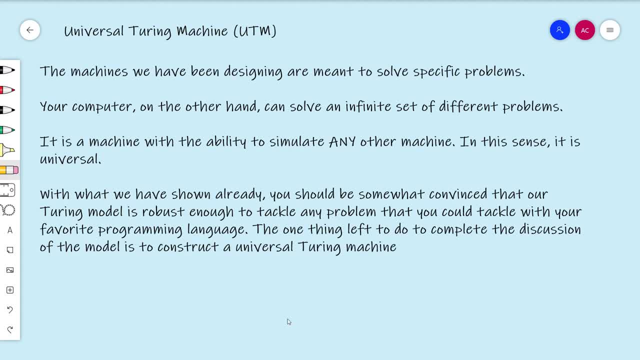 this machine probably still kind of seems weaker to you than what you typically view as a computer. Now why is that? Well, the reason for that is that your computer is very special in that what we think of as modern computers- the computer in front of me and the computer in front of you- 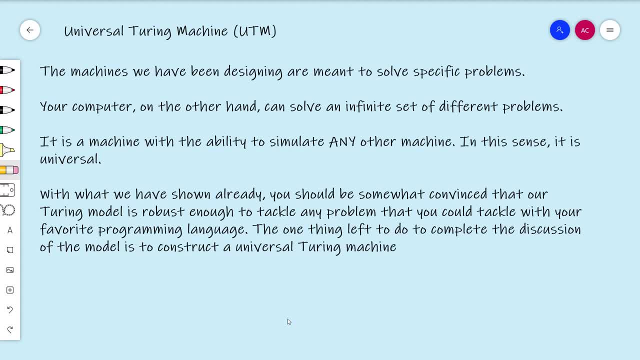 these are special machines that are with the capability of simulating other machines. This computer you're running a program, an operating system that has the ability to simulate other machines. It has the potential to run potentially any other program, any other machine. 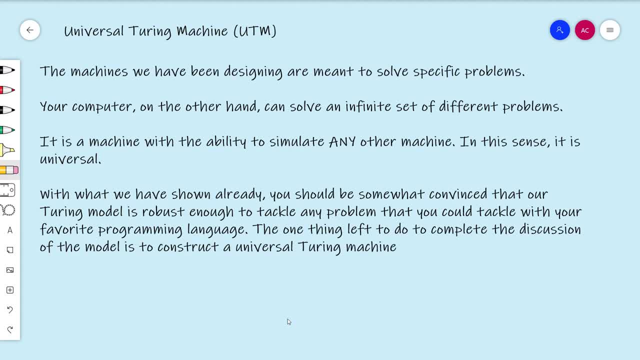 What you have in front of you is a machine that can simulate other machines. The machines that we've been making so far are machines that solve very specific problems. I make a problem to solve the palindrome problem. I make a machine to add two numbers. 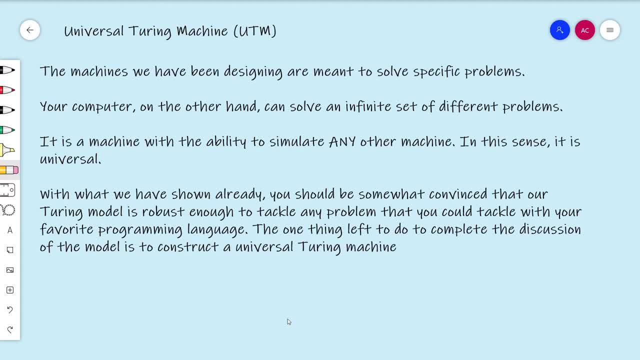 I make a machine to do this or do that. I make a machine to do something specific, But the machines that you're used to thinking of as computers are kind of more powerful than that. They can simulate anything. They can simulate any of those machines that we've been talking about. 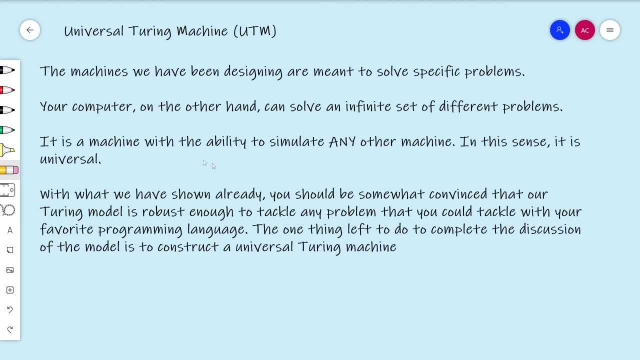 And that's what I mean by universal. A universal machine is a machine that can simulate other machines within its model, And in some sense this is as much the standard bearer of a competent model of computation as its ability to solve problems. You kind of have a competent model of computation. 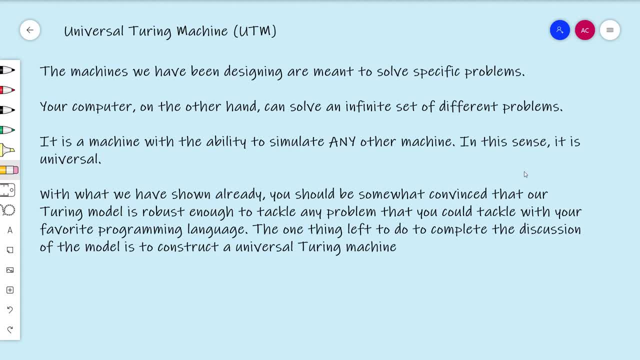 If your model of computation is sophisticated enough that you can build out of it a particular example of something that can run other machines in the model, You can have a really competent model of computation if you can build a universal machine in your model. So that's what we need to do. 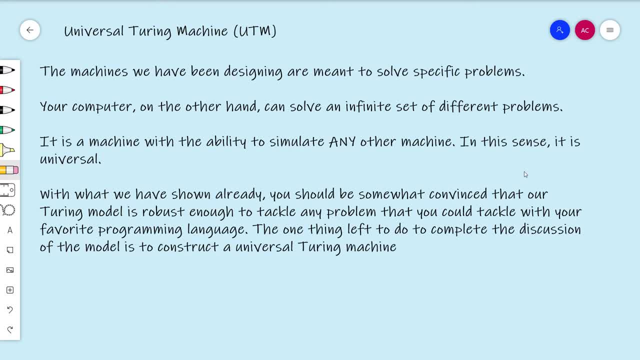 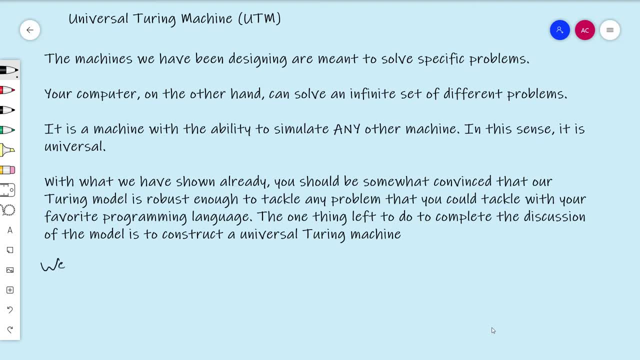 In order to kind of convince you that we have a fully developed model of computation, we really need to create a universal Turing machine. So we will denote our universal Turing machine And what I'll usually write is UTM, U, The machine. U is going to be a machine that takes two inputs. 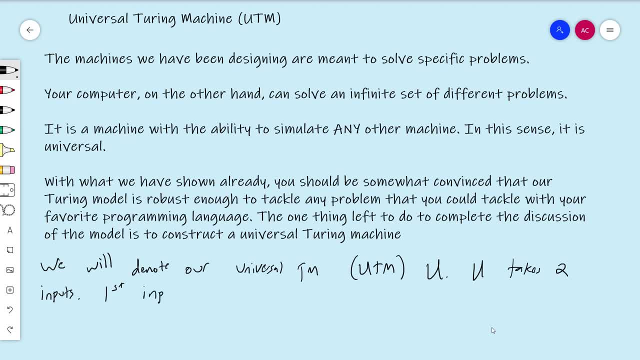 First, the first input is another machine- I'll call it M- And the second is an input to M. It's an input to that machine. It takes a machine and then it takes an input to that machine. It is an input to that machine. 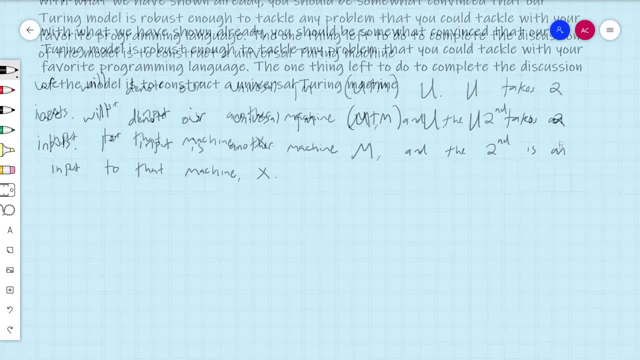 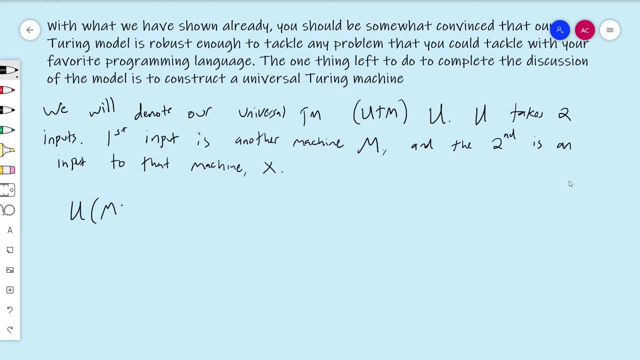 I'll call it X And so basically what a universal Turing machine is going to do. The defining kind of idea of a universal Turing machine is that U of M I'll put like. I mean I'll put like a. Usually you put like a comma in between inputs. 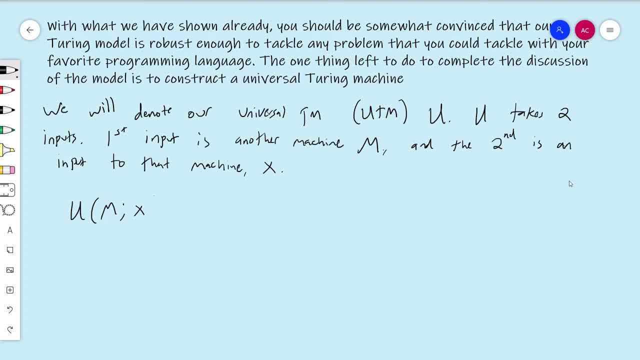 But this is a very big input, So just separate it out. I'll put like a semicolon, But it's really just M comma X is equal to M of X. So what it does is U takes a machine and an input And what it does is it simulates the machine M on that input X. 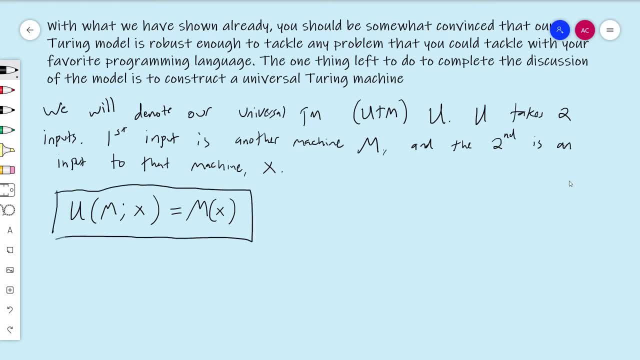 This is what it means to be a universal Turing machine. So obviously there's kind of a bit of a weird thing going on here, right. But what is the input to a Turing machine? in general, The input to a Turing machine is a string. 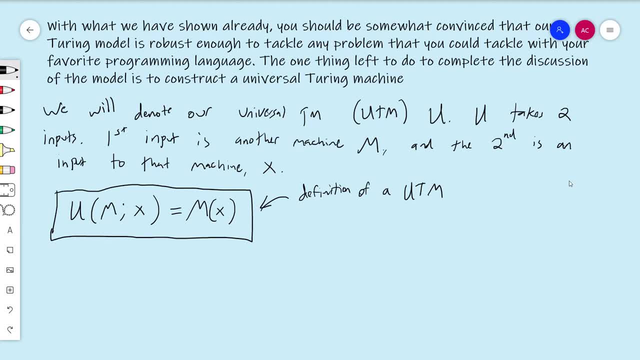 But I've sort of broken that convention here. I've said the input to this Turing machine is a string X, But then another Turing machine. A Turing machine isn't a string, is it? Well, no, it isn't. So what we really need is we need to find a way to encode a Turing machine description as a string. 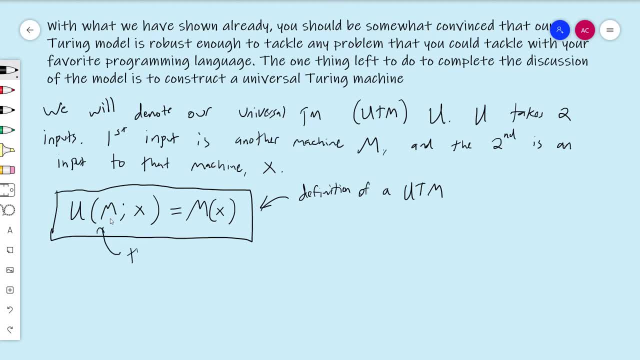 So, in a way, this is going to be a string, This will be. This is really a string, Representing the complete description of a Turing machine, And you should think of it as a program, right? What this really is is it's a set of characters. 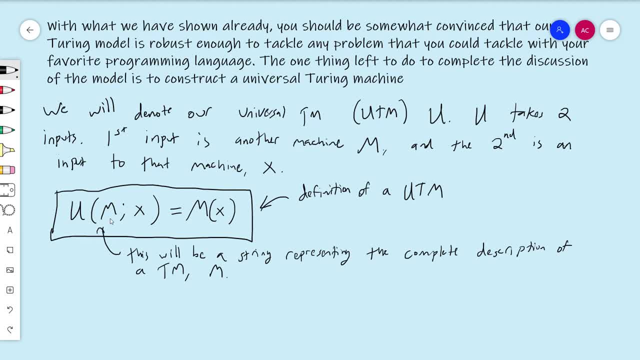 It's a big string that represents a machine, a computational process, And so this is really the way that you think about it. This is a. You should think of this as a program. You should think of it as a program. So what this computer takes is it takes a program. 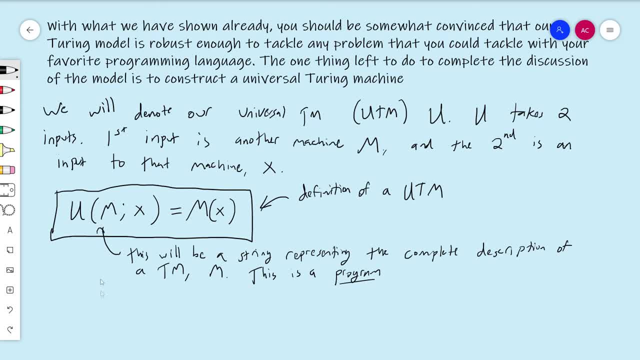 I've written a program in some language that is the language of Turing machines, And then I've given an input to that program. So you should think of this as the program. What we need now is What we need is a standard. We need a standard method of how to do this. 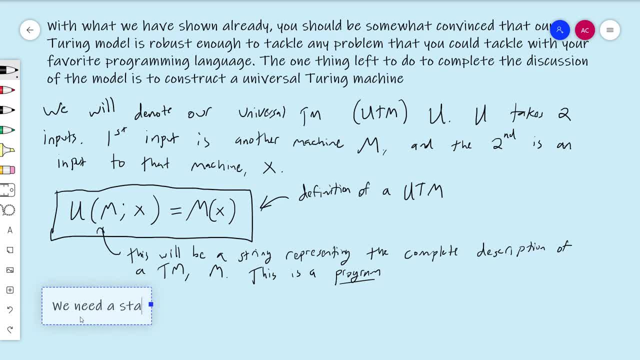 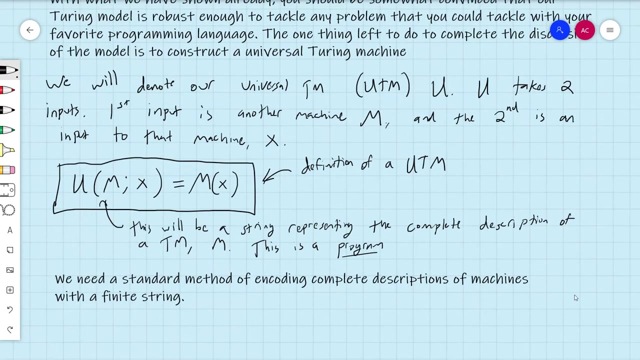 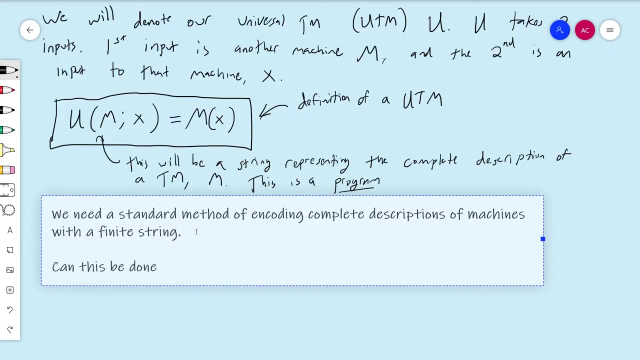 So we need a standard method of encoding complete descriptions of machines with a finite string. So, first of all, can we do that? Well, of course we can. So can this be done? Certainly, And I think you can believe that, but it's something that I haven't talked about yet. 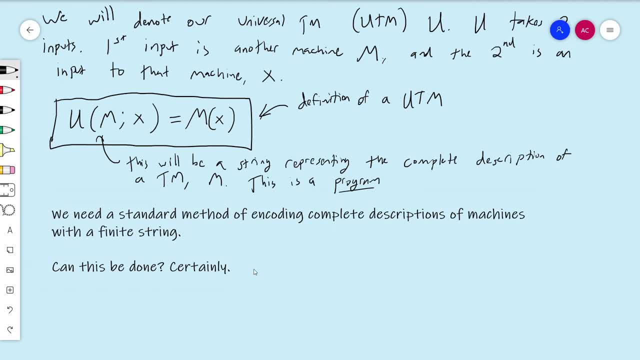 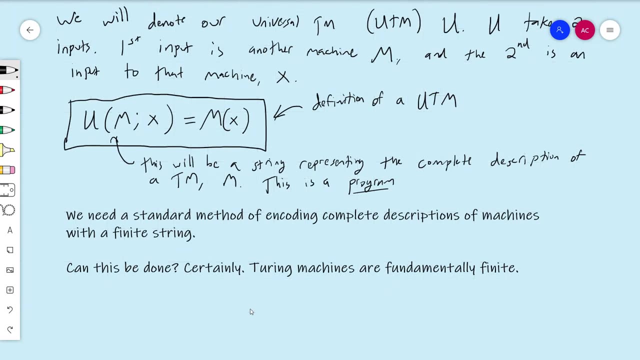 And it's incredibly important, And so this is a good time for me to talk about it. You know, Turing machines are fundamentally finite, in the sense that I can describe them in a finite way. I mean, I've given you, I've written down lots of Turing machines. 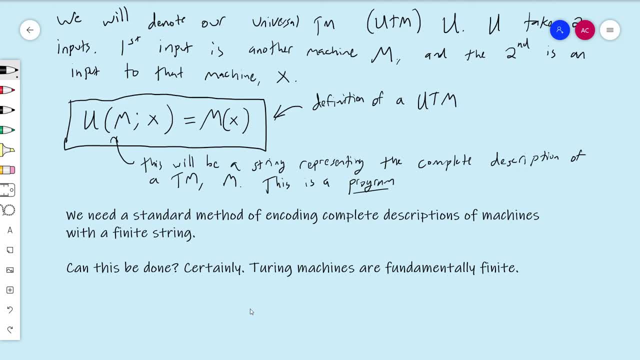 like the complete description of lots of Turing machines at this point. Right, Just think about the palindrome problem. How do we give you, How do we make a Turing machine for the palindrome problem? I wrote down on my screen everything involved in it. 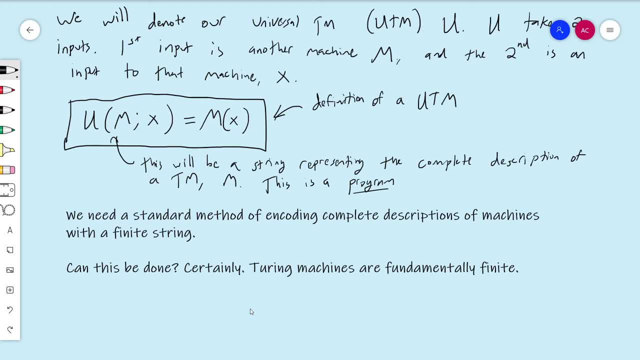 and everything involved. I also gave you a complete Turing machine. when I was giving you that Turing machine that did the space-creating subroutine right, That was. I just gave you a table And just We can kind of think about it right. 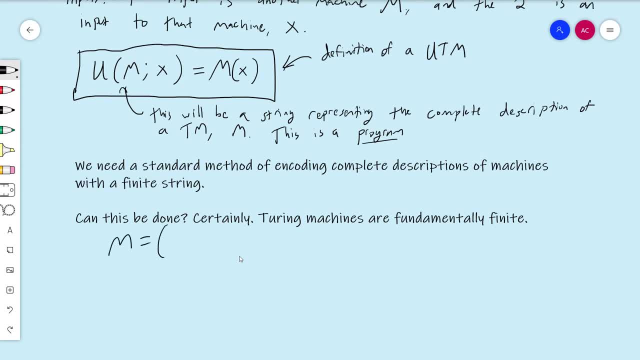 Like if you have in a machine M which is sigma Q, delta, this thing is finite, This is a finite set of characters, This is a finite set of states. And then this thing: this is a little more complicated, but it's a function. 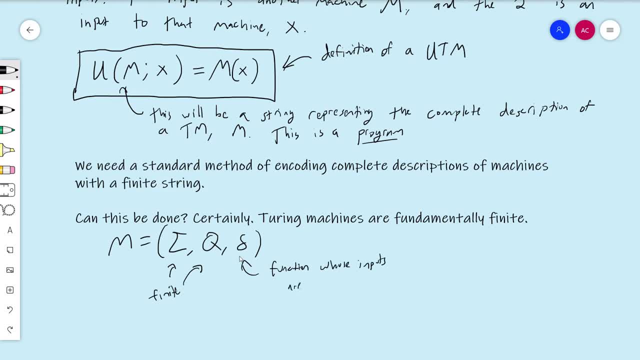 whose inputs are sigma state, You know are symbol-state pairs, And so as a function, you know, you can completely define a function by just completely defining what it does at each of the inputs. And so how many inputs are there? 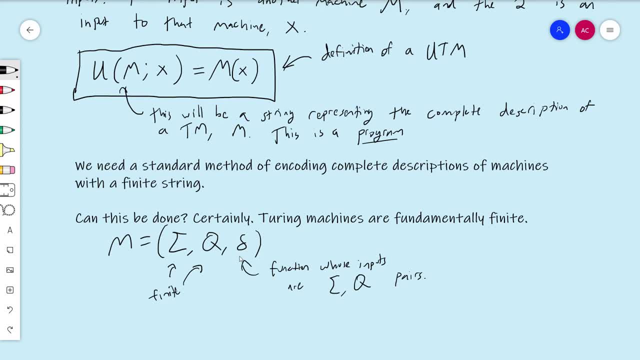 Well, there's this many times this many. Sorry, There's this many times this many. So So the transition function is just a finite list as well. It's a finite list of function inputs and outputs. So this whole thing, this is a very finite description. 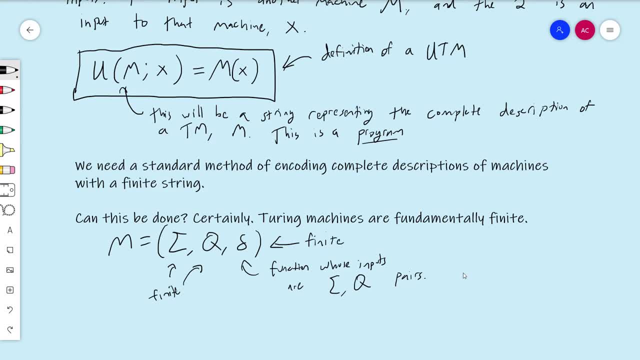 This is kind of itself a finite description. I just need a way to standardize how I'm going to represent it as a string in some alphabet. But fundamentally this is already a finite description. And think about what it does, right? A Turing machine. 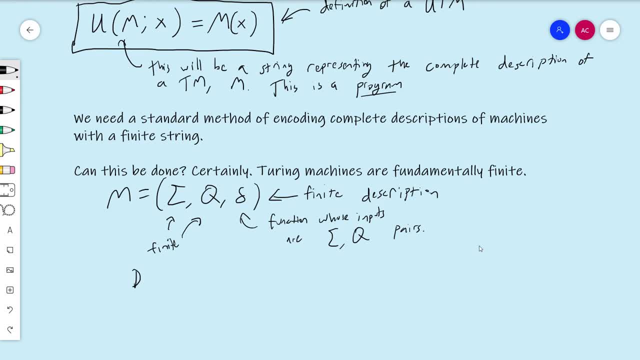 despite being finite, a Turing machine decides a language which is infinite. So what it does, what a Turing machine really is, is in kind of a more like linguistic sense. So a Turing machine is in some kind of fundamental sense, in a kind of foundational way. 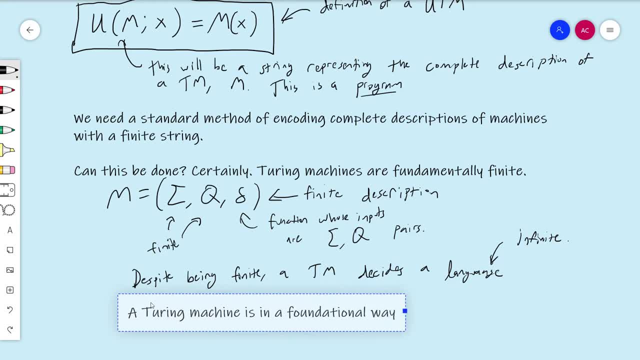 kind of to divorce what we've been doing kind of from computability entirely, is to say that a Turing machine really what it is is: it's a finite description Of an infinite set. It's an infinite set that I'm specifying in a finite way. 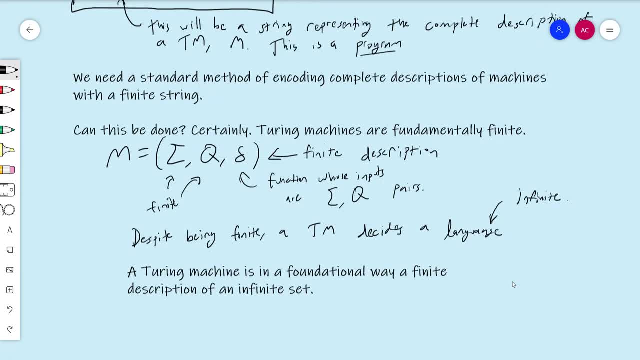 I have a problem and if I have a Turing machine that halts on every input, that specifies a set, that completely describes an infinite set in a finite way, So that's kind of what a Turing machine kind of is, in kind of a divorced sense from computability theory. 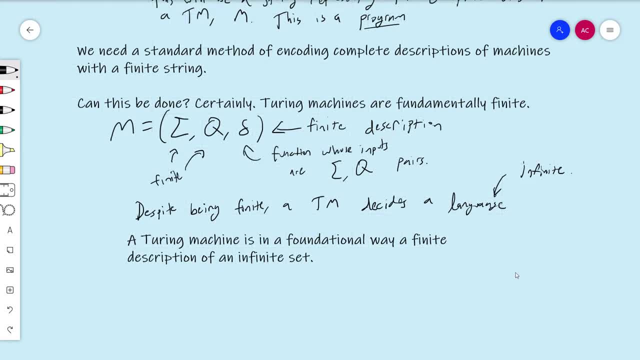 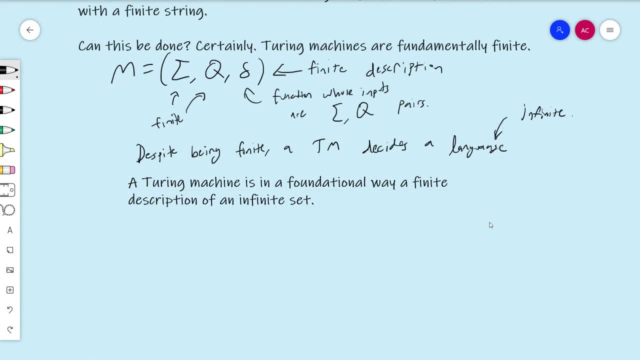 To what extent can I describe a language within a finite way, And so that's kind of deeply connected to Turing machines. So, anyway, what we need to do now is just kind of standardize it for the sake of creating our Turing machine. So the alphabet. 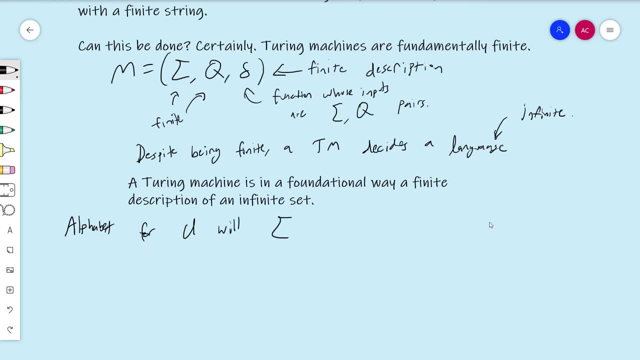 for U. we're going to make it this: It's going to have a 0 and a 1, so we're just going to have our binary kind of alphabet stuff. It'll have our typical triangle. it'll have a blank symbol. 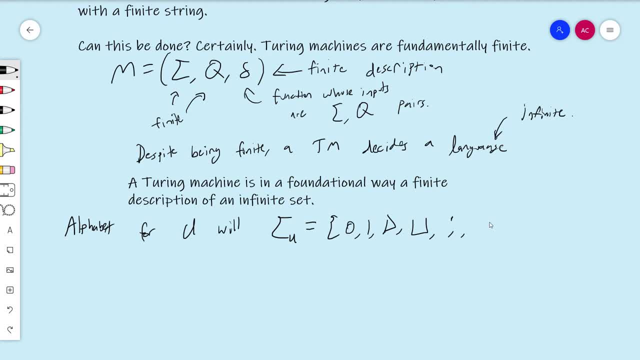 and it'll have a semicolon. it'll have a semicolon as well, and it'll also have parentheses and it'll even have a comma. So it looks kind of weird because I'm separating out the symbols by commas, but this comma. 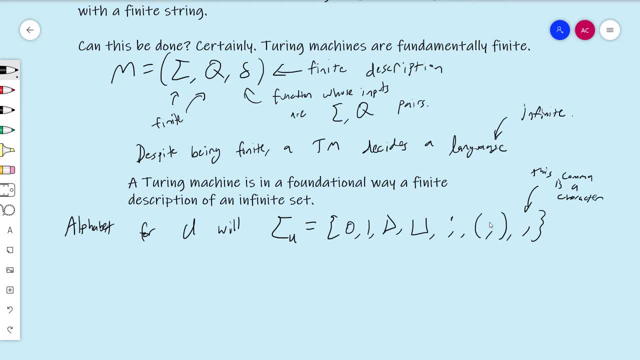 is a character in the alphabet. So I mean, this is our alphabet and we're at that point where I can just kind of say I can just kind of make my alphabet whatever is convenient and this is really the convenient alphabet. 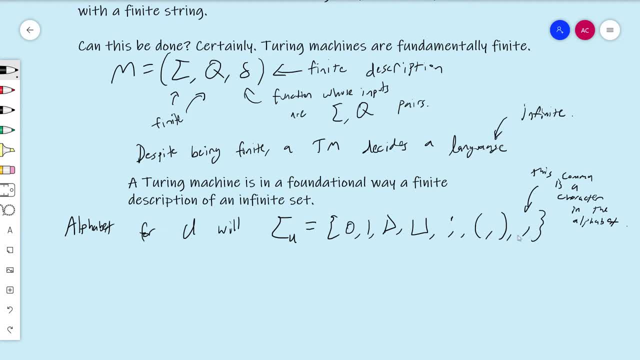 Parentheses are convenient, so I'm going to throw them in. Commas are convenient, so I'm going to throw them in. At this point, I can do that because I've proven equivalence between different alphabets Now. that said, 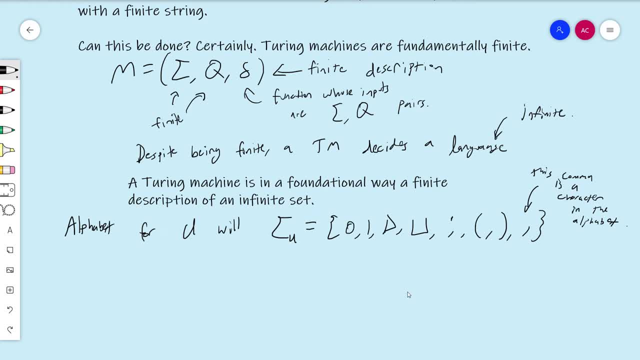 the alphabet for M. on the other hand, for M is going to be any number of characters And I don't necessarily have to do this. You know, I could build a universal turning machine for the set of turning machines over a fixed alphabet. 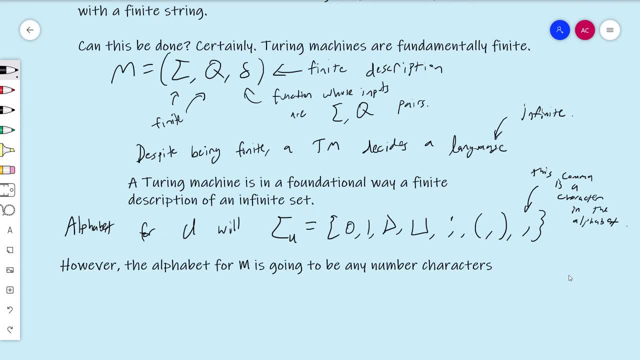 and that would be just as kind of that would be just as good of a proof. but it's not that much harder to make a turning machine that works over any finite alphabet and I think that would be more kind of impressive to the viewer. 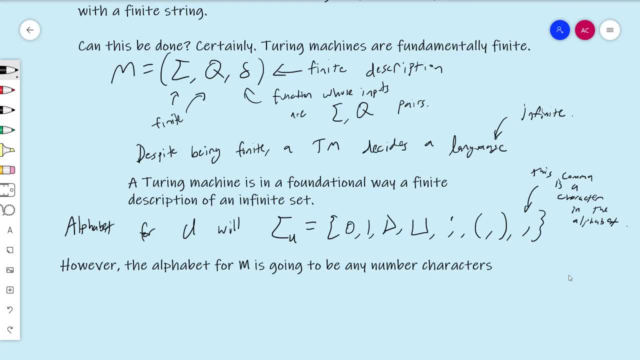 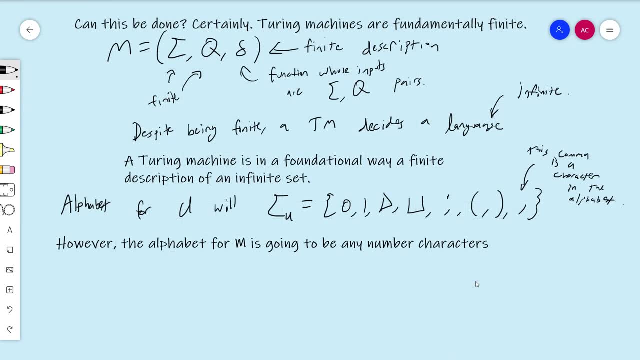 And so I'm going to do it like that. I'm going to have M be an arbitrary sized alphabet, even though I know I could just kind of take whatever M I want, collapse it down to two symbols if I wanted to, and then assume every turning machine input. 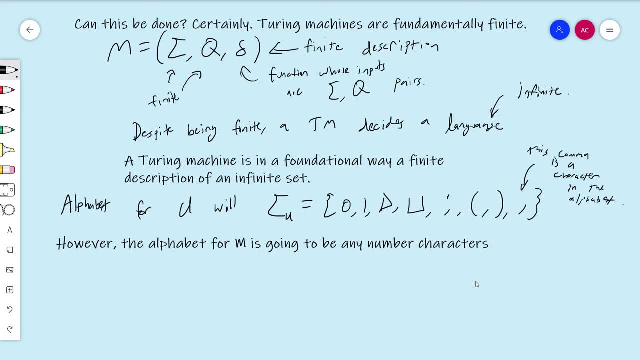 has two symbols in their alphabet. but I won't do that. I'll assume it has any number of characters. but what I will assume is that the characters are all kind of from the same set and that they're signified. So the turning machines can be any number of characters. 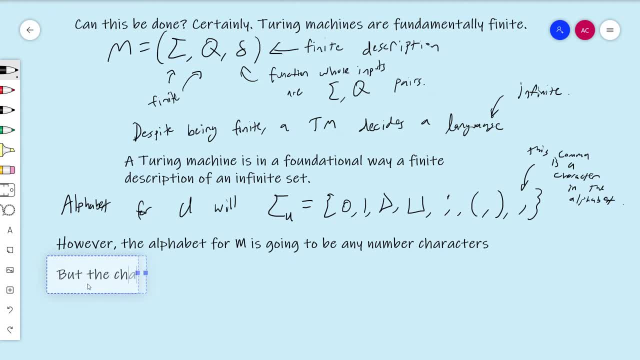 but the characters are all from some common set of characters, some common infinite set of characters. Like maybe take ASCII- right, ASCII's got tons of characters, so maybe all of our turning machines use characters in ASCII. You know, maybe it uses twelve of them. 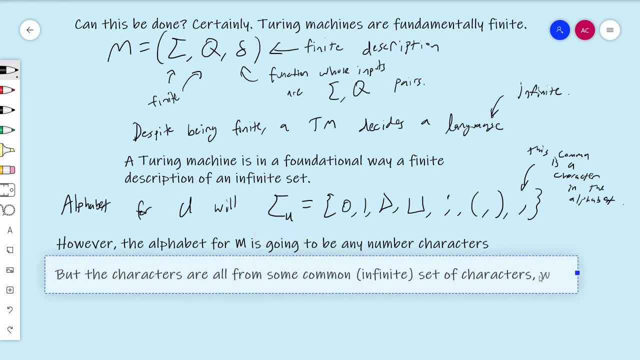 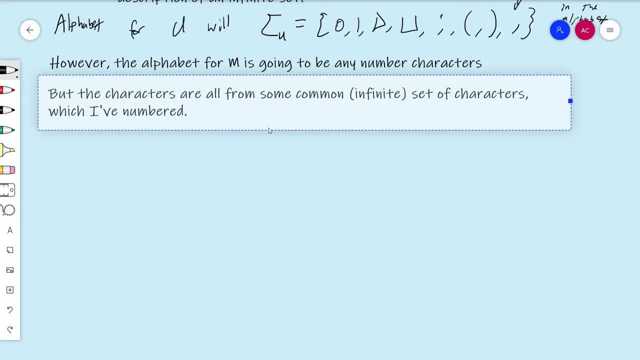 maybe it uses eight of them, but it uses some characters from this common set which I've numbered. And in addition to that I'm also going to assume that the states of the turning machine will be from the same set. So states for any turning machine. 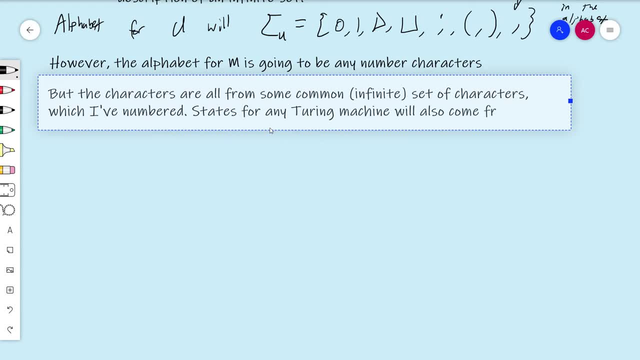 will also come from this set. So I mean I need symbols for the states as much as I need symbols for the characters. They serve a different purpose, but they can come from the same infinite set. It doesn't really matter what they are. 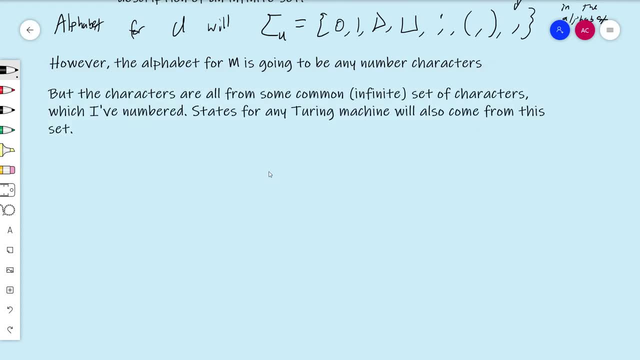 And so the idea is going to be that you know, let's say that my turning machine, you know, let's say that my infinite set, big set of characters, is, I don't know, maybe like just the English alphabet. 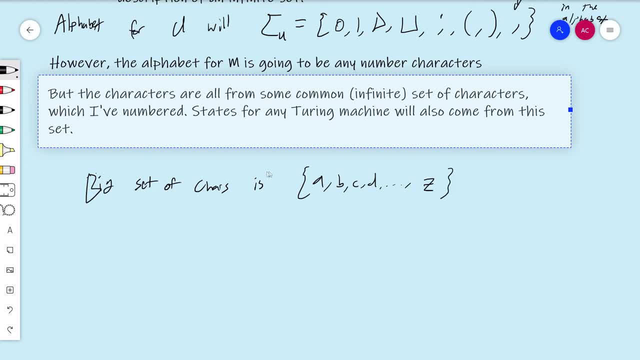 Up to Z right. So there's an implicit numbering of these characters. This is obviously not an infinite set, So just maybe, like you know, let's just suppose that it continues forever somehow with other symbols, If my turning machine's alphabet 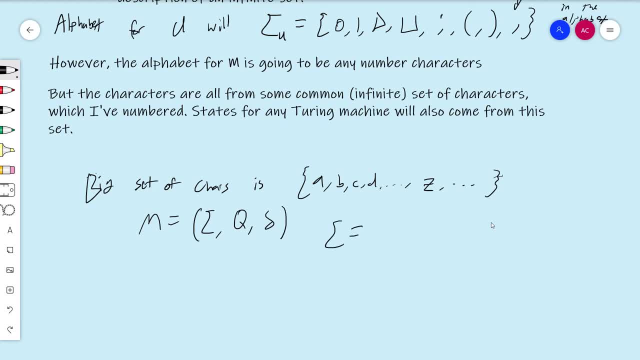 If my turning machine's alphabet is like, let's say, just I don't know- D, F and L, you know, it doesn't necessarily have to be the first three. I'm just going to pretend that it's the first three symbols. 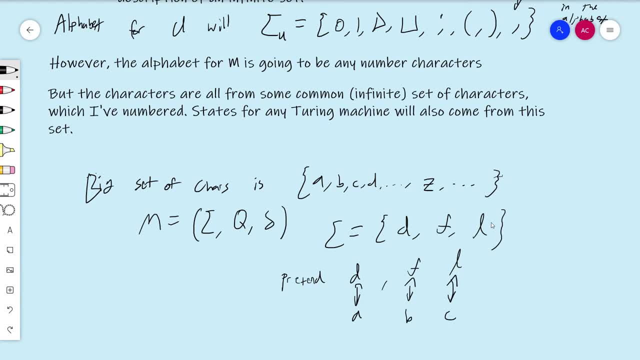 You know. the bottom line is: if the alphabet is three symbols, I can. There's no harm in pretending that it's the first three symbols, right? So I'm just going to pretend that Ds are As, Fs are Bs and Ls are Cs. 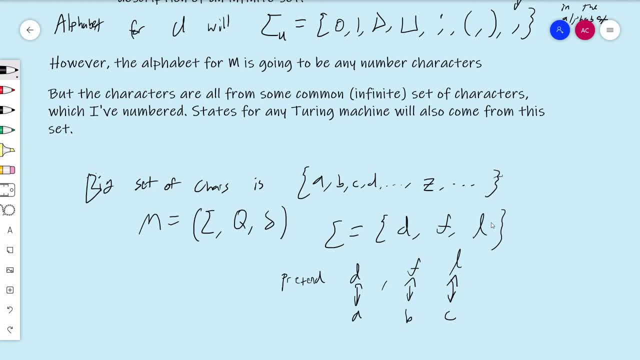 And so because of that, I can, Instead of thinking about the symbols at all, I can think of. Instead of thinking about it as ABC or D, F, L, I can think of it just as one, two, three. And so, in fact, by doing this, 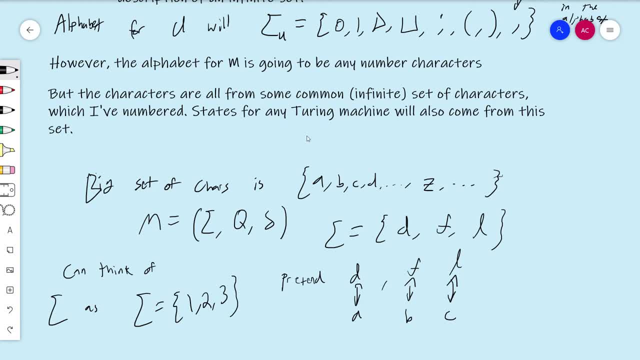 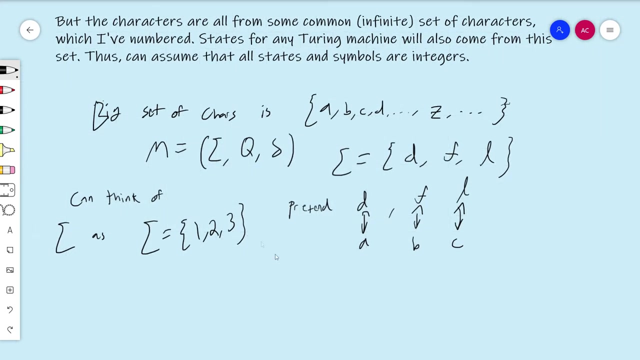 I can assume that all of the states and symbols are integers, More or less right. They're integers that represent symbols, But they're specified by integers And so also one other convention I'm going to say is that you know. 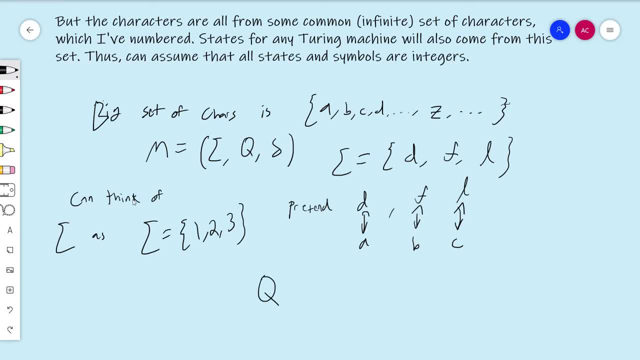 let's say that the states for M- Remember the states and symbols- are all coming from the same set. So if the states of M are like B and Z or whatever, let's say there's only two. I'm going to assume that. 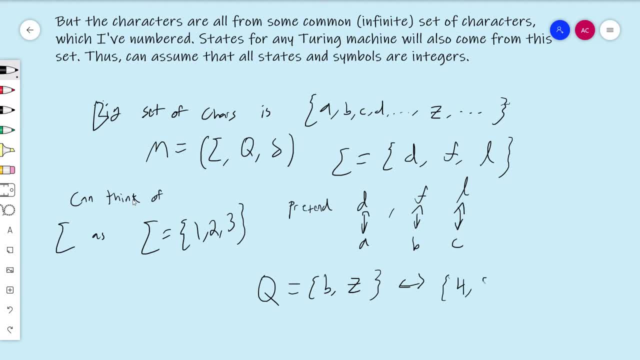 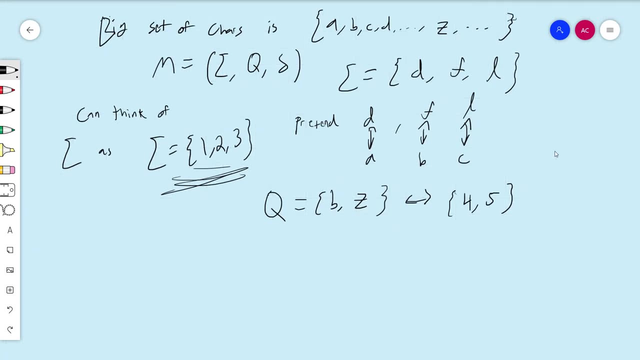 instead it's going to be four and five. So not only is it still going in the order, it's going from the order, continuing from this. So let me summarize that The idea is that, So, if M is equal to sigma Q, delta. 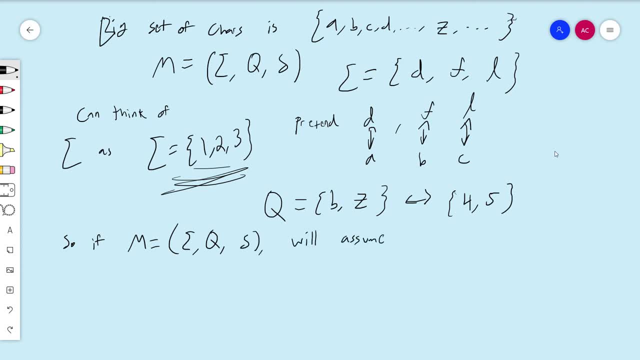 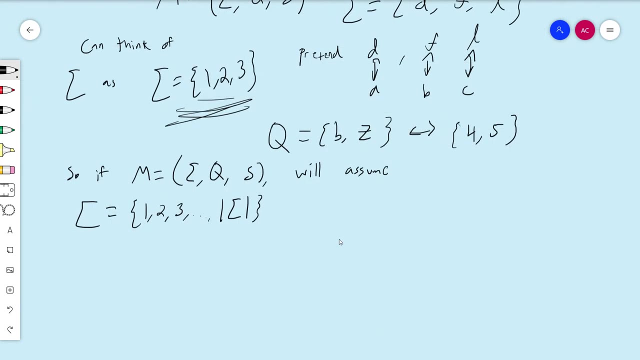 we'll assume that sigma is equal to one, two, three, dot, dot, dot up to the size of sigma, And what I mean by that. By the way, I've done this a few times, I've said this before. 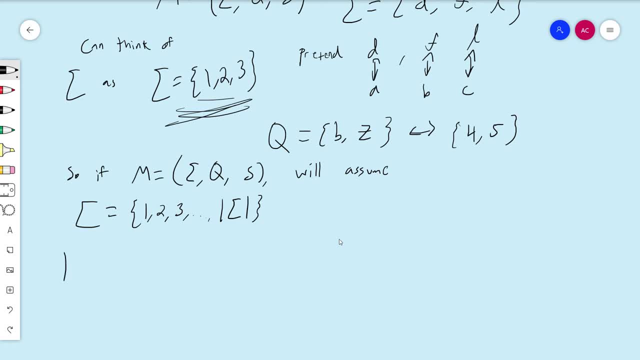 I've used these bars a bunch of times without explaining it. When I put bars around a set, I mean the number of elements. So if I put bars around a set, I'm referring to its cardinality, that is, the number of things inside of it. 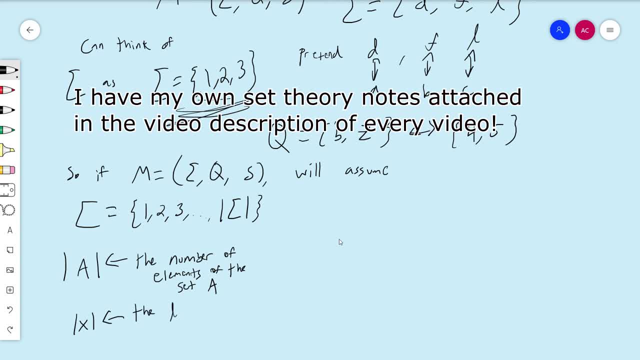 And if I put bars around a string, I'm referring to the length of the string. I've done this a bunch of times. I've used these bars all over the place and I've kind of hoped that I think people have probably seen these bars. 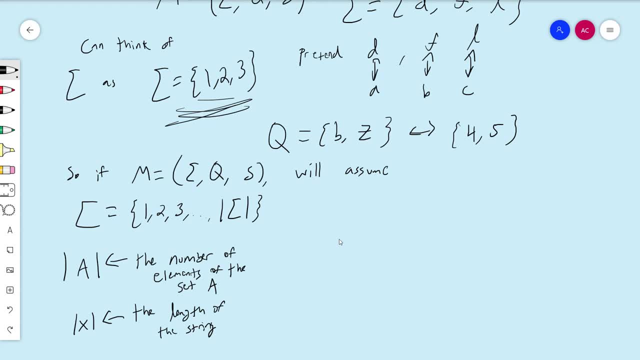 and gotten an understanding of what I mean by them. but I felt like I should say it explicitly. You know, if you put bars around objects in math in general, you're referring to kind of their magnitude, kind of in some sense. 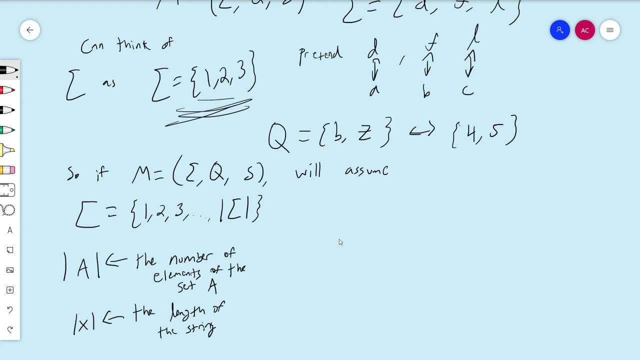 The exact nature of what magnitude means for the object is sort of context-sensitive, depending on what you're putting bars around. But you know you can see a number of things in a set length of a string. These are very related ideas. 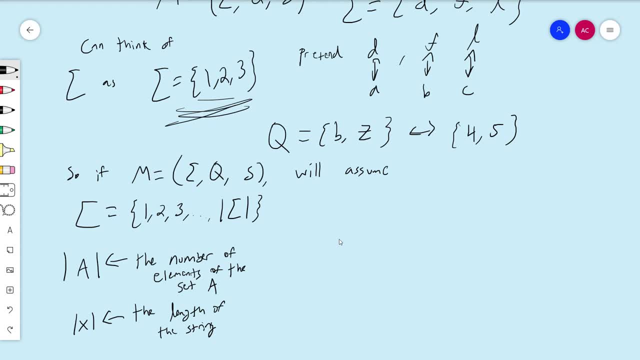 They're kind of size, So, anyway, that's what I mean. So when I say sigma is equal to 1,, 2,, 3, up to sigma, I mean it's 1,, 2,, 3,, dot, dot, dot up to. 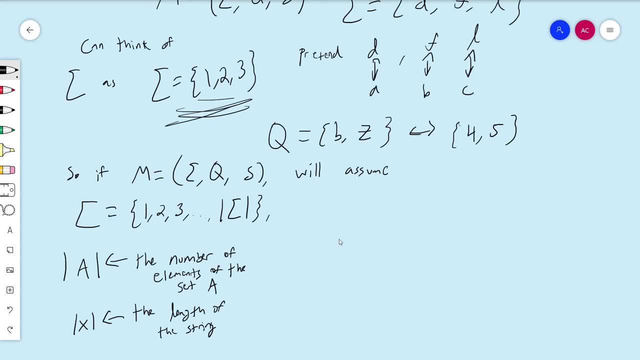 just however many things are inside of it. Also, then, q is equal to. It's going to start counting up from however many things are in here, So it'll be sigma size plus 1, sigma size plus 2, dot, dot, dot up to sigma size. 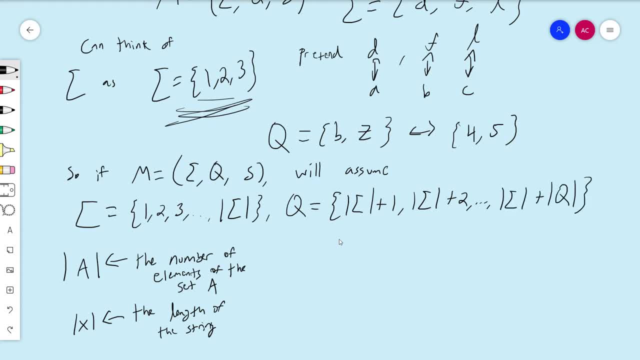 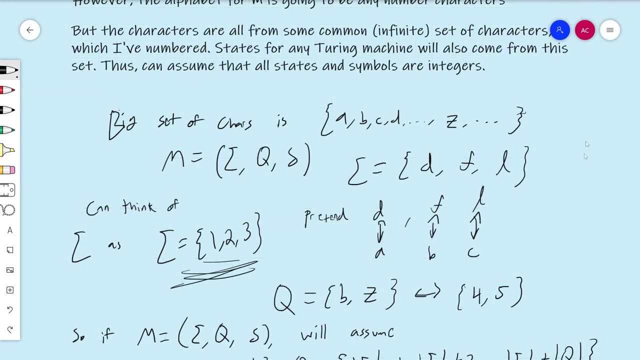 plus, however, many things are actually in q, So this is going to be my standard. Finally, Oh wait, there's a couple more things. Finally, Remember, my complete description for a Turing machine is going to need to include symbols, obviously, and states. 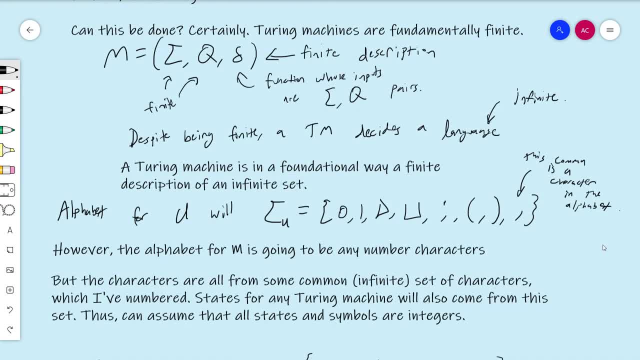 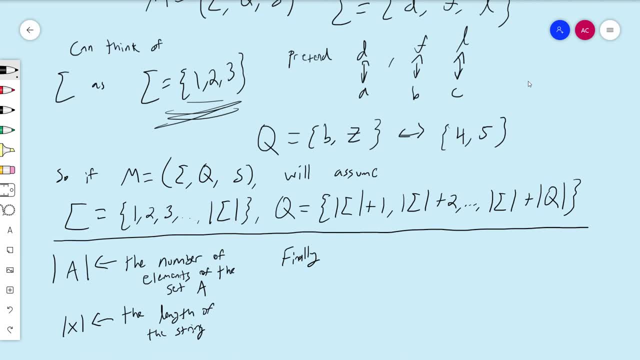 but it's also going to need to include: Remember this delta function also spits out directions, and there's three of them, so I need three more symbols to denote the directions, And so, finally, sigma plus q plus 1 and sigma plus q plus 2. 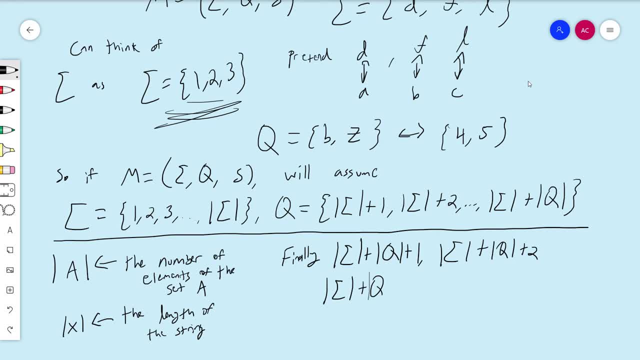 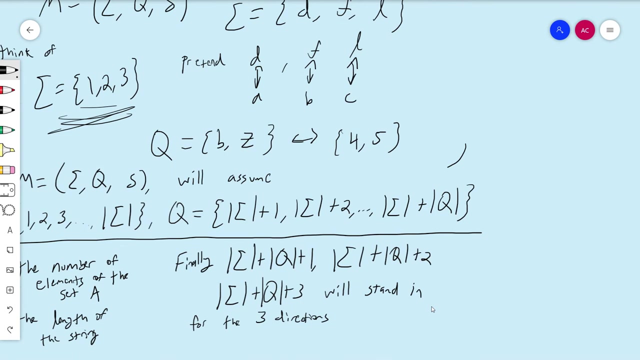 and sigma plus q plus 3 will stand in for the three directions That a cursor can go. So, And then also Wait, one more bit of convention: Sigma plus 1.. I'll always interpret sigma plus 1. Maybe I'll just put it here, actually. 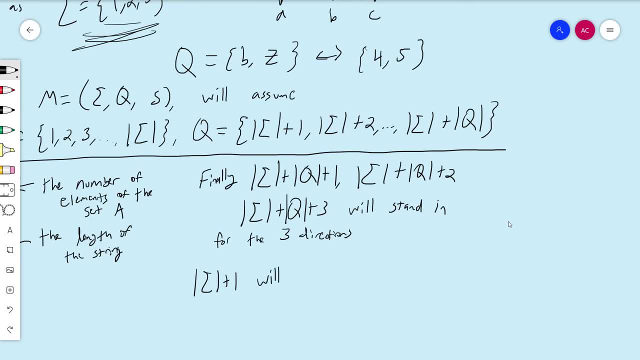 Sigma plus 1 will always be the initial state And the last three numbers in q will always be the halting states, Right, the acceptance state, the rejection state and the actual just ordinary halting state respectively. I'll always assume that those are the last three states. 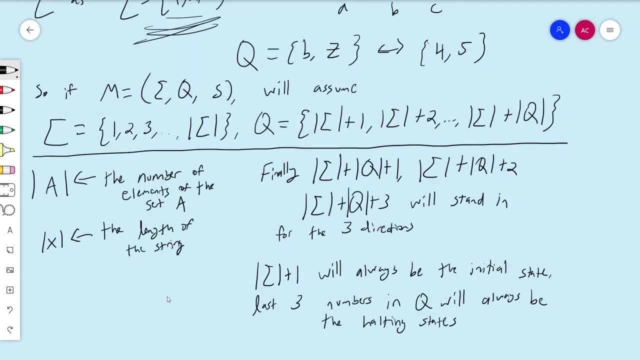 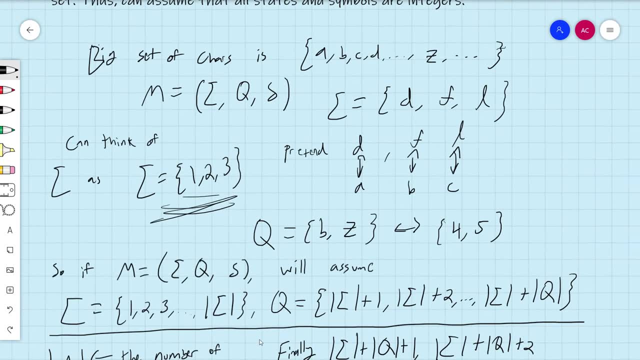 So that's kind of like. Finally, I've sort of fully specified, I think, everything I need to, And of course you know, integers are integers. but my Universal Turing Machine alphabet doesn't have integers. It has 0 and 1. It only has two of them. 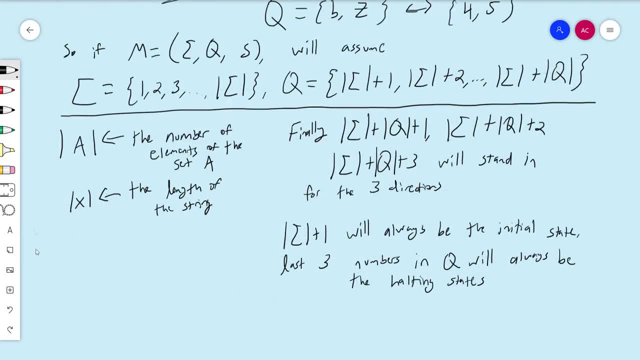 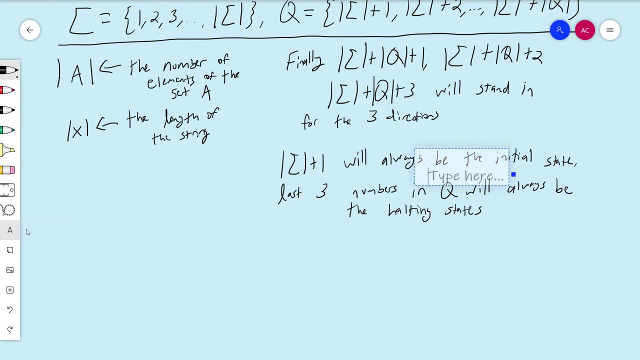 So what I'm going to need to do is represent them in binary. So, So all of these integers will be represented in binary, Using a certain number of bits, Depending on sigma, and q In particular. if you remember that video that I did on the codings of alphabets, 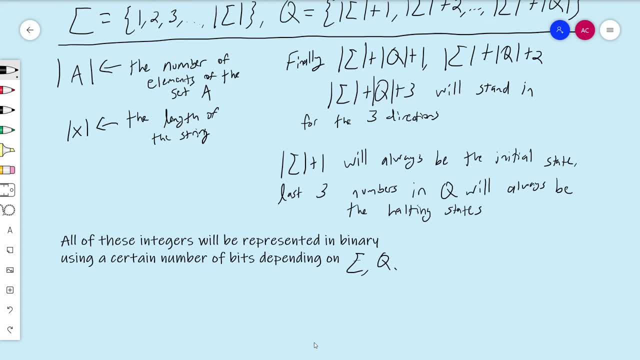 you'll remember that the number of bits that I'm going to need, that is, the number of symbols that I need to denote a single integer, is going to be log base 2 of the size of sigma plus the size of q plus 3.. 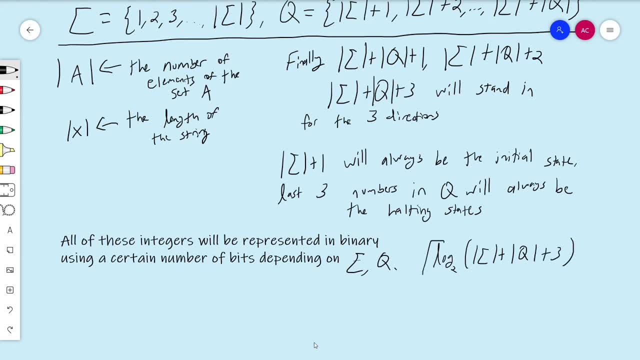 That is the number of symbols, total, the ceiling of that. This many bits. And you know I didn't completely spell out how to count in binary or do a conversion to binary in that video, But the idea is really simple, right. 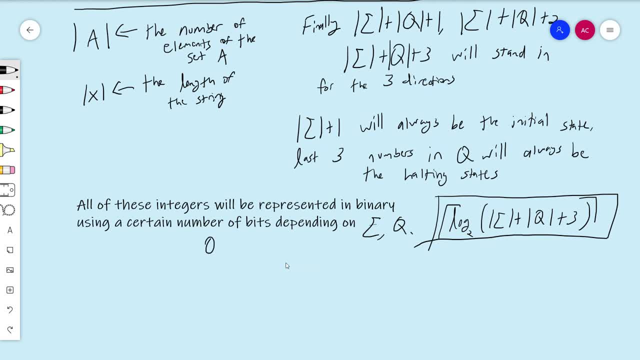 If I you know, I'll start with 0.. How many characters do I have to represent all the integers? I have 2.. 0 and 1.. So I'll start counting. So 0 is what I'll call 0.. 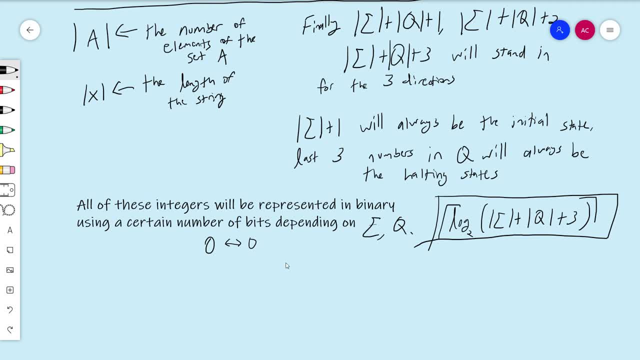 And I'm not going to write down all of the correspondences, But after that I'll have 1.. That'll be 1.. And now I'm out of symbols So I have to kind of Now I have to use 2 kind of characters. 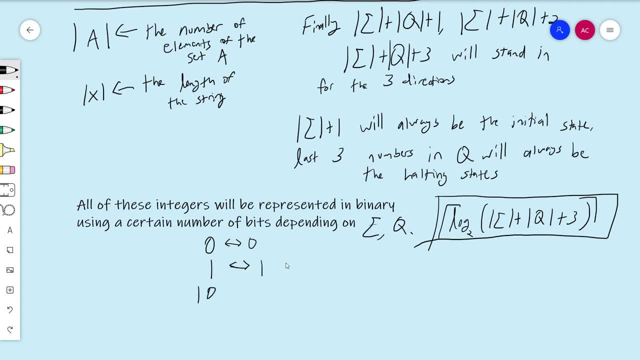 Now I have to say: Now I'll say 1, 0.. This'll be 2.. Right, So I just kind of start over the 0 count, I start over counting in this, I start over counting in like the 1's place. 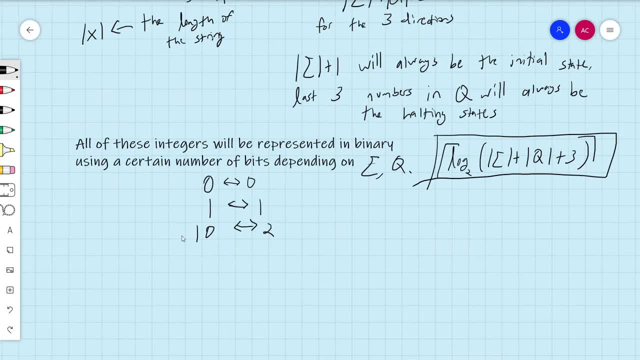 And now I start counting in the 2's place, Where, you know, usually this would be called the 10's place, But since I'm counting in binary, this is now the 2's place, And then this'll be the 4's place. 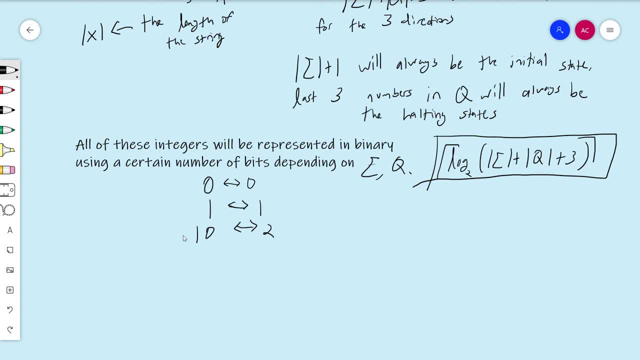 So you know this is how you count in binary: You go 0,, 1, and then you reset. You put a 1 over here: 1, 0.. 1, 1.. Now you're out of room in both these slots. 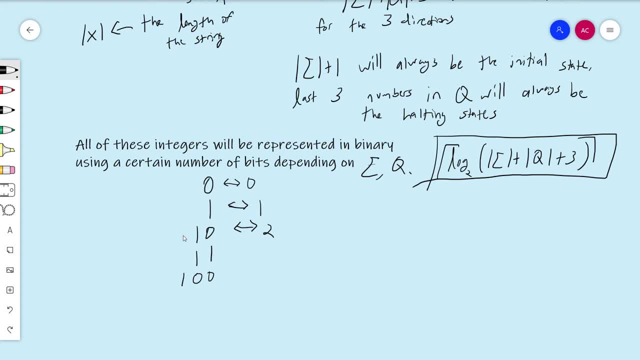 Now you move over here: 1, 0, 0. And then you restart the process with 2 bits here: 1, 0, 1.. 1, 1, 0.. 1, 1, 1.. 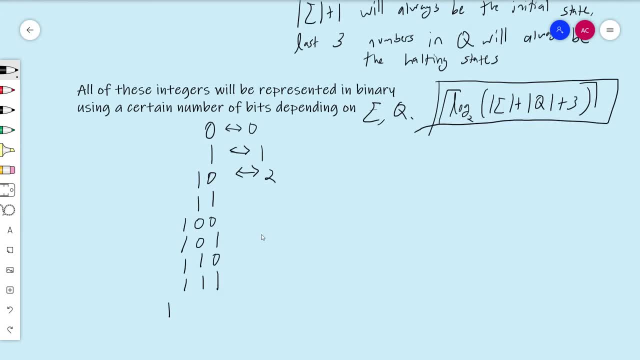 And then you're out of space again, And now you move over to the. Well, let's count. This is a 3.. This is a 4.. 5,, 6,, 7., And so this'll be the 8's place. 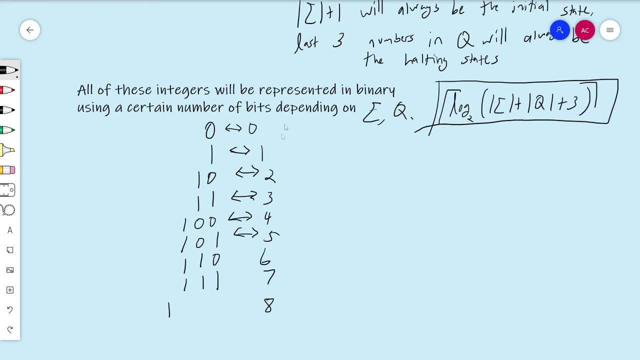 And, if you notice, that's 2 to the 3rd. So this is the 1's place. still, The 1's place is always the 1's place. The 2's place is what would normally be the 10's place. 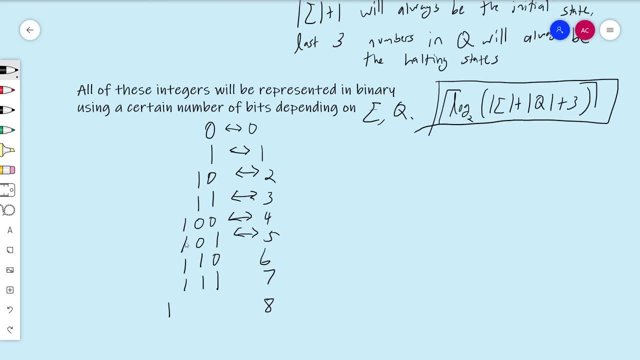 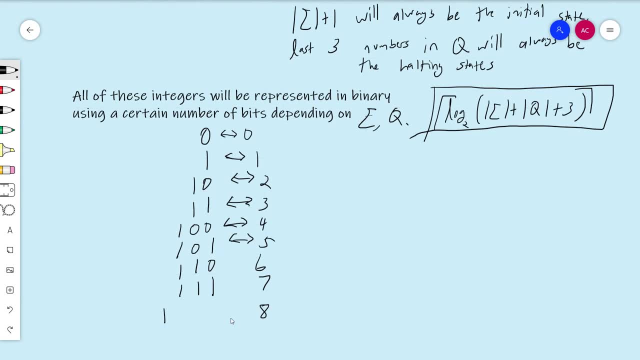 The 100's place is now the 4th's place, The 1000's place is now the 8's place, And so on and so forth. But this is how you count in binary. It's really simple. Now we want all of them to be the same length. 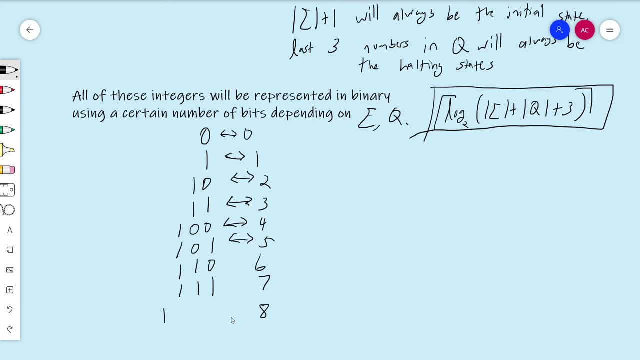 This is the number of bits we'll need, That is, this is the number of places, The number of place values that we need to represent this many bits. So what I'm going to do is I'm going to pad with leading 0's. 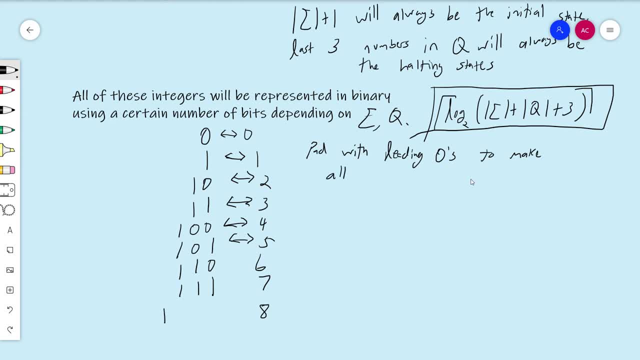 to make all binary representations the same length. So I mean I'll put like, if I need 4 bits, then I'll put like 0's, like this. I talked about this kind of thing in my coding's video, But definitely worth reviewing, especially since that's my least. 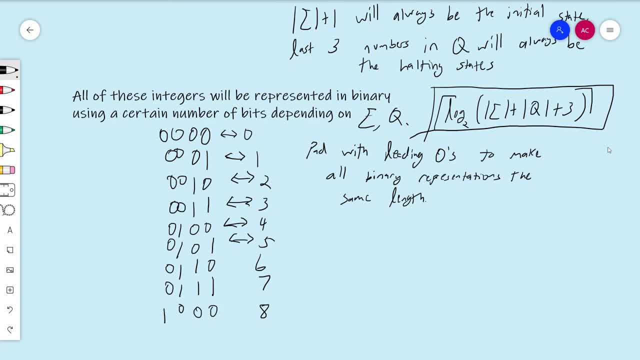 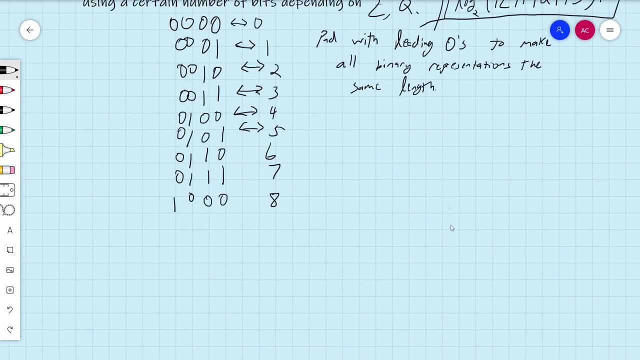 I think that's the least viewed video in this whole series so far. So that's what that is. So everything will be the same length. Then it'll be able to. So basically, if I can just specify the size of these two sets, 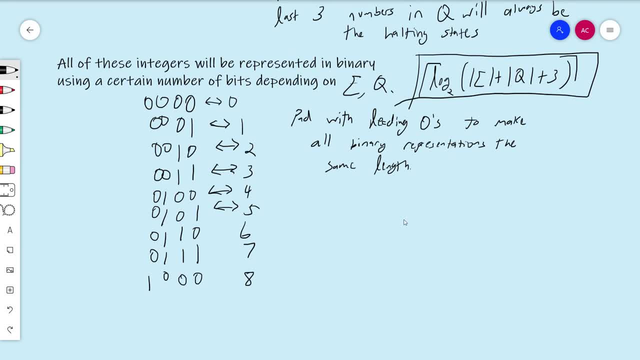 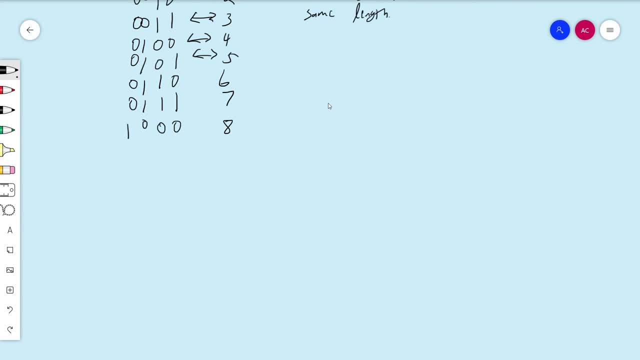 then I've fully specified sigma and q. So now let's talk about the actual description of m. So the description of m will be 3 strings separated by commas. First will be the size of the. So this is the first guy. 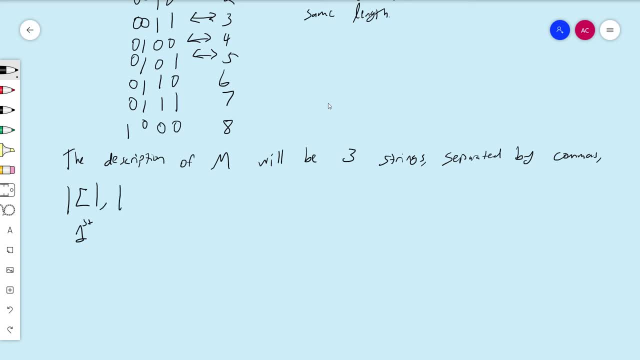 which is the size of the alphabet, and then a comma, and then the size of the states. And so note that these two things, if I just start out with these two things, these two numbers, in binary mind you, these two numbers. 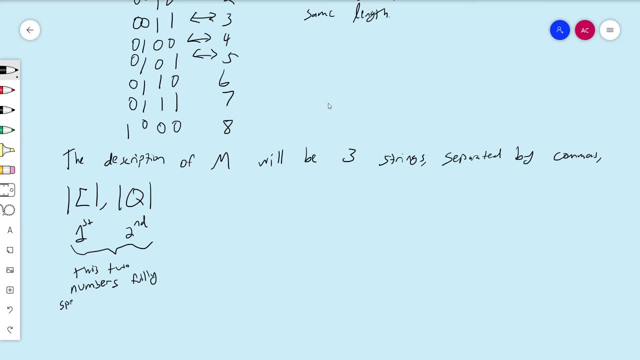 fully specify the set of states and the set of symbols. If I just give you these two numbers by my convention, I've actually given you the entire alphabet and the entire set of states. The only thing that's left still is a description. 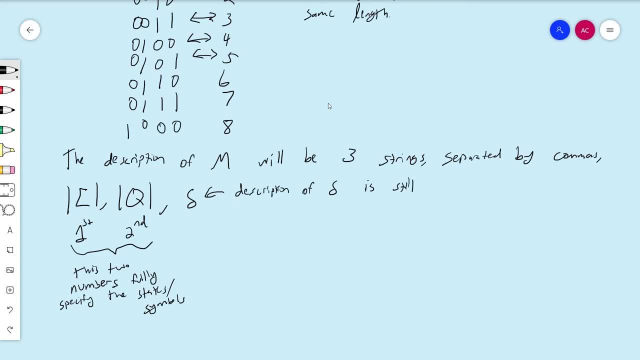 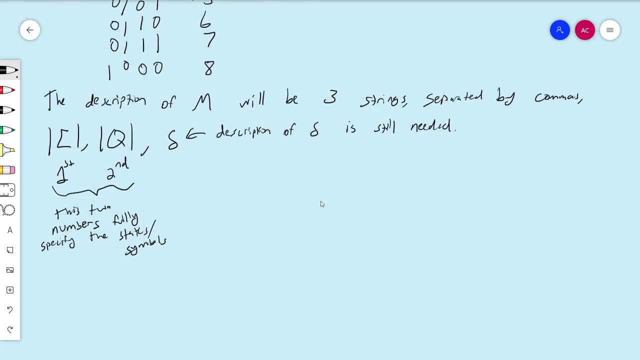 of the transition function is still needed. So how do I do that? How do I describe the transition function? Well, the transition function, remember, is kind of a table. It's kind of a set of inputs and outputs, But I can always represent it as kind of. 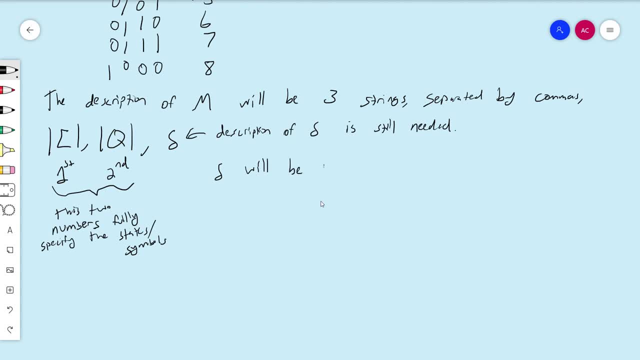 So delta will be represented by a set of pairs of the form. It'll look like this: So there'll be like a sigma and a p Or a sigma and a q I guess I usually start with for some reason. 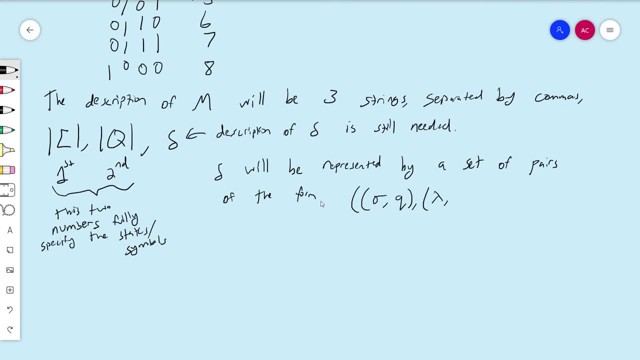 And then it'll be another triple over here. It'll be a lambda and a p and a delta and a d. So it'll be two parentheses. And remember parentheses and commas are part of my Universal Turing Machine's alphabet. 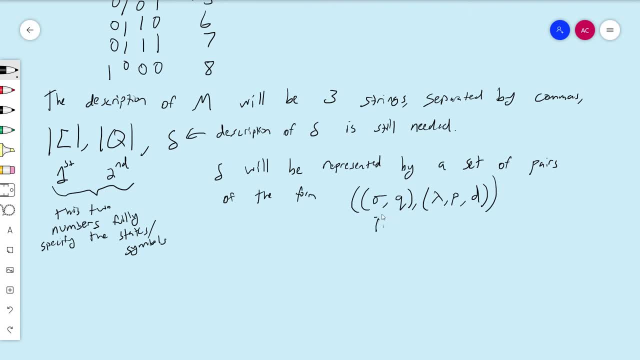 And then these guys. these are symbols and states and directions. These are all, of course, represented in binary And you know conceptually, because my description of this Turing Machine leads with sigma and q, the Turing Machine will be able to do a calculation. 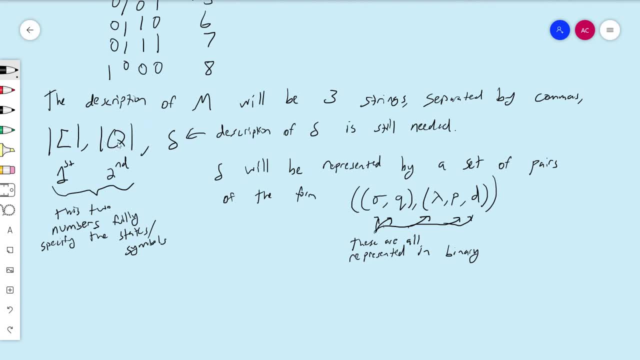 and then figure out from these two numbers that I'm given, which are separated by commas, how many characters the binary representations of things in delta are going to be. So it will make that calculation and then it can move over here and figure out like 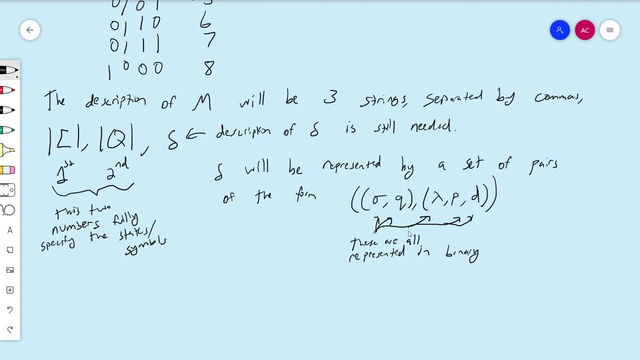 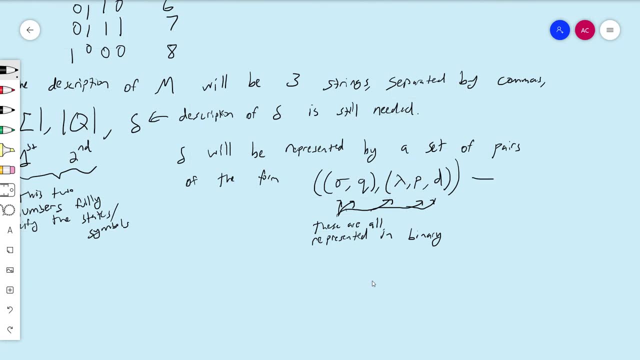 okay, I need to go this far to get to the state from the symbol, and then it knows all of that stuff. These are represented in binary And, of course, what does this represent actually? This corresponds to the instruction that the function delta of sigma and q. 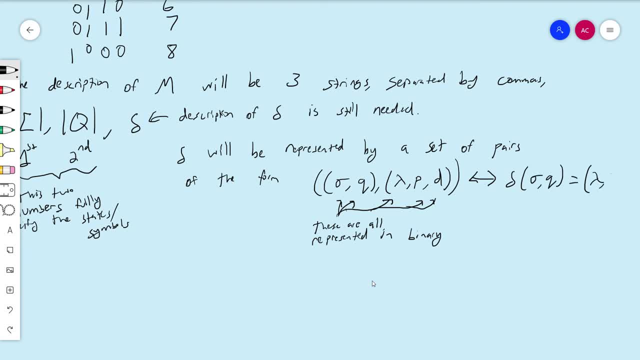 is equal to lambda p, d, So. So that's what this represents. So if I just basically It'll be a set of all of these, It'll be a set of all the instructions represented this way, surrounded by commas. 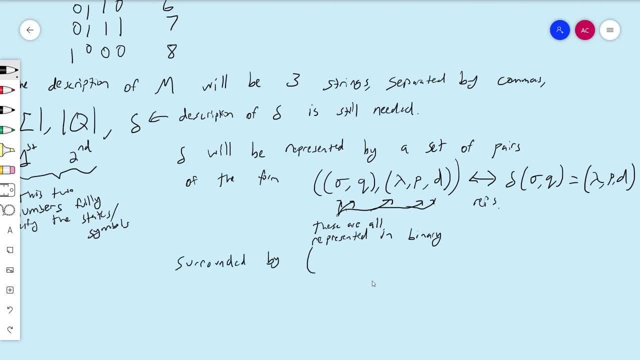 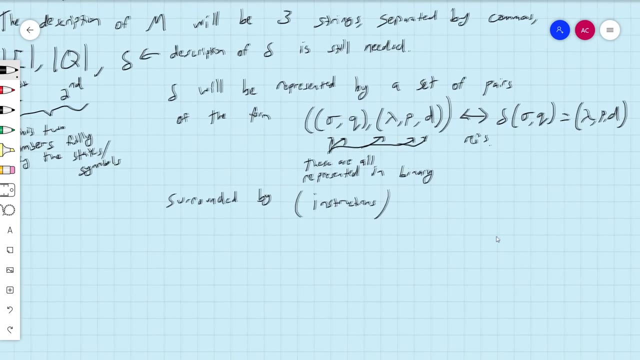 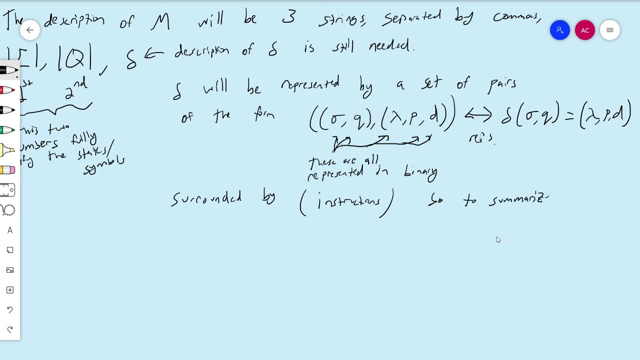 Surrounded by parentheses. I mean So the whole set. So it'll be like this: and then instructions in this form here and then another parentheses, So to summarize, And that's the full description. So to summarize, M is going to look like this: 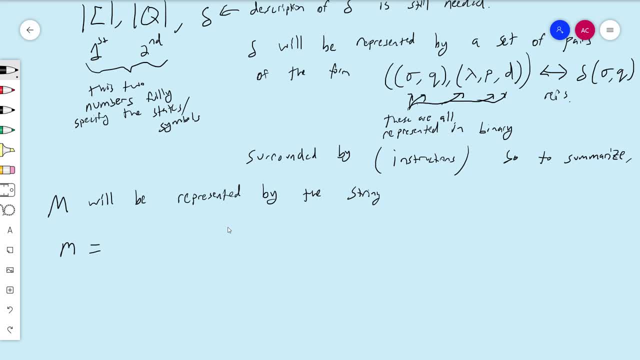 I'll use little m just to make a distinction between the actual Turing machine and the program that represents the Turing machine. the string: It'll be size of sigma comma, size of q comma, and then it'll be a big parentheses. 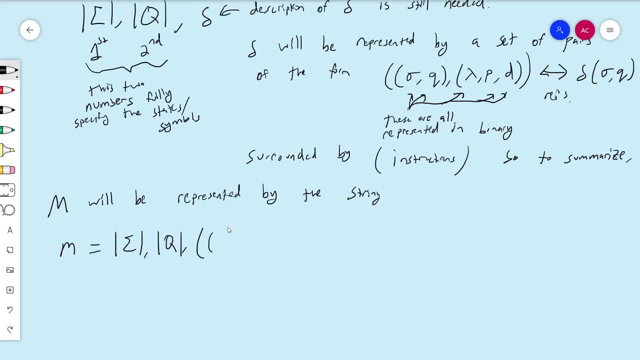 and then another, and then it'll be the pairs like this, So it'll be like: Maybe I'll just put Like: these'll be numbers, so it'll be like one, and then, I don't know, like eight. 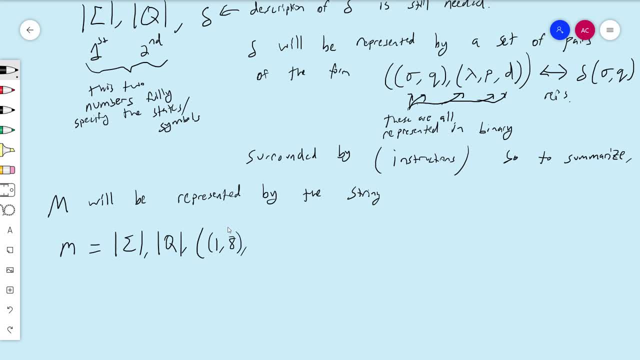 and then it'll be in here, delta of one, Whatever that is. Yeah, Yeah. so this is one object, and then another one would be like I don't know, two, twelve Dot, dot, dot, And then finally, the last one I'll imagine will be: 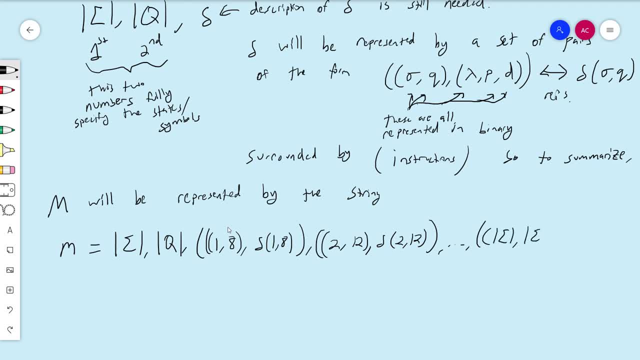 you know, size of sigma, size of sigma plus q, comma, delta of that stuff, It'll look like this. So the complete set. So it's long. I mean it's a long string, but this is a program. 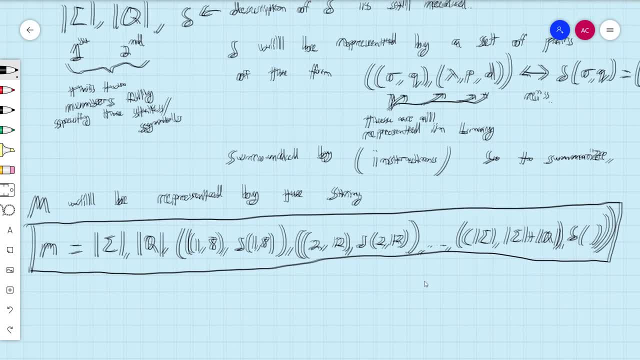 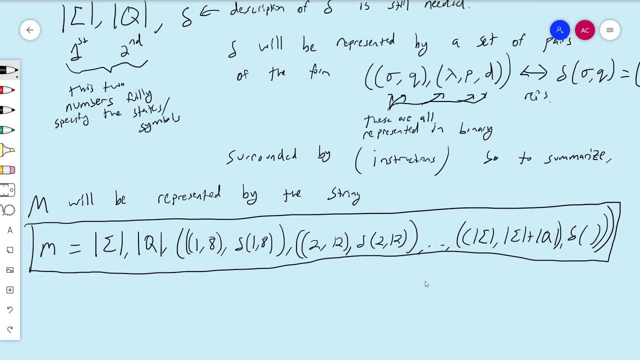 You can see how this is a program. So this is our standard. This is how we're gonna represent a Turing machine, And every Turing machine represents this way, And maybe, as an exercise, you should think to yourself: don't try to make a Turing machine for it. 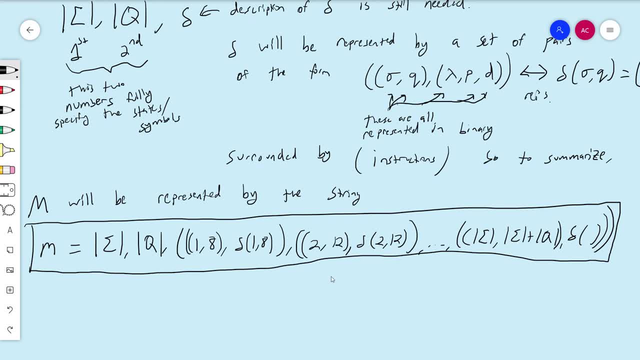 but write down an algorithm, for Maybe I'll write this as an exercise And, by the way, I'm rerecording this. This is like I've already made the videos past this and I actually kind of skip the step in which this needs to be done. 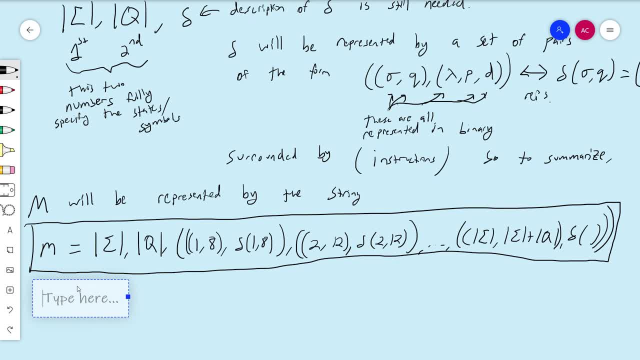 but this is kind of the first step, necessarily, of how to make a universal Turing machine Exercise. Describe an algorithm for deciding if a given string codes a valid Turing machine. So I'm giving you a string and I'm asking you, does it code a valid Turing machine? 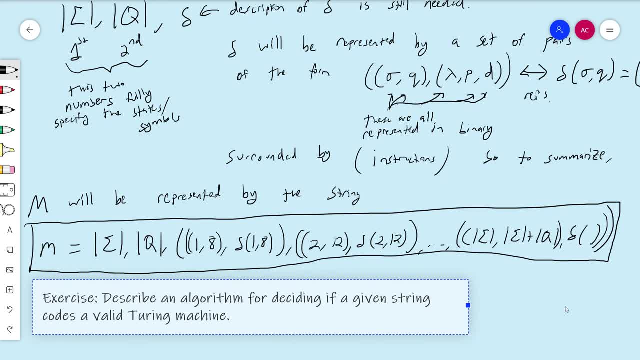 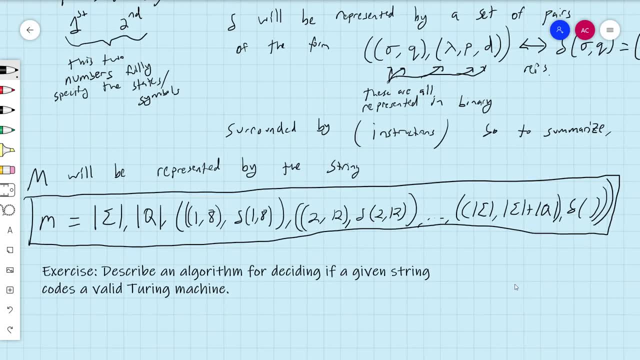 in the sense that does it represent a Turing machine in this form. So you don't have to do this exercise. I'm just giving it as exercise more or less, because I mean it's kind of worth thinking about, but also I'm giving it. 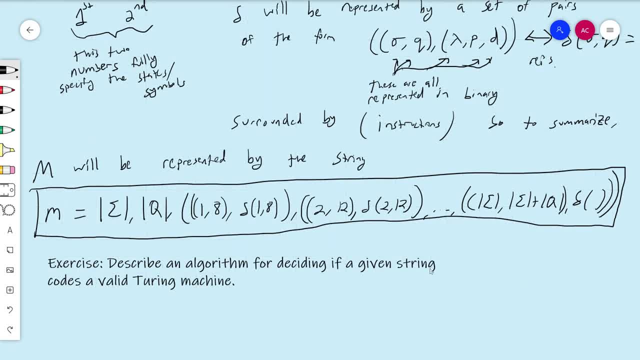 because I didn't feel like thinking about it in my proof. that follows this. so Technically you do need an algorithm for this, But my hint to you is that you first need to calculate the logarithm of this plus this plus three. 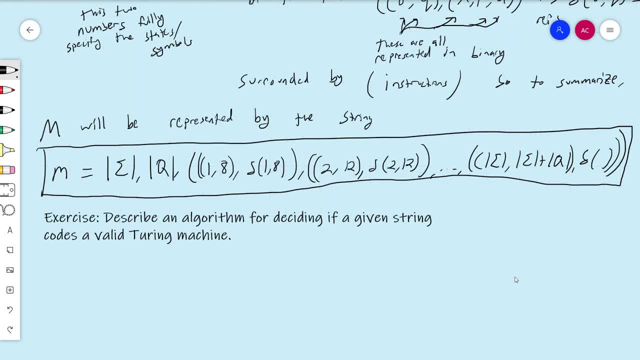 That's what you need to do first, But anyway, that's our convention.